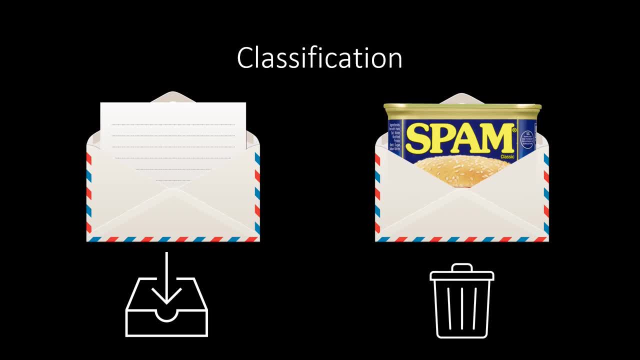 The spam classifier has two possible outcomes for any given input email. Either the email is classified as spam or it is considered legitimate. In other words, overall there are four possible combinations. We have two actual input classes: legit email or spam. 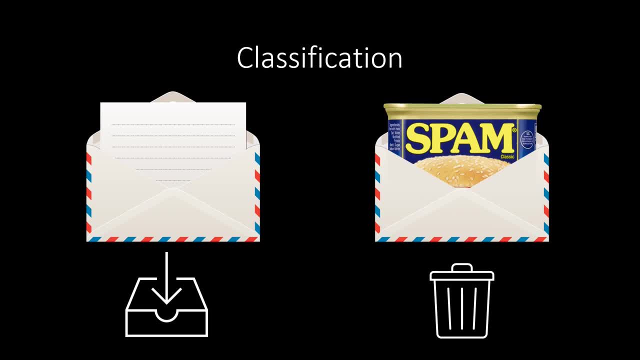 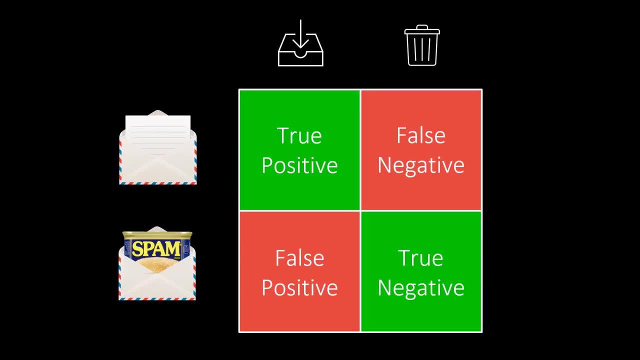 And we have two possible classifications: let the email pass or delete it. We can naturally visualize these four combinations in a two-by-two matrix. The two rows are the true types and the two columns are the predictions of the email classified. The two green cells of the matrix are desired outcomes. 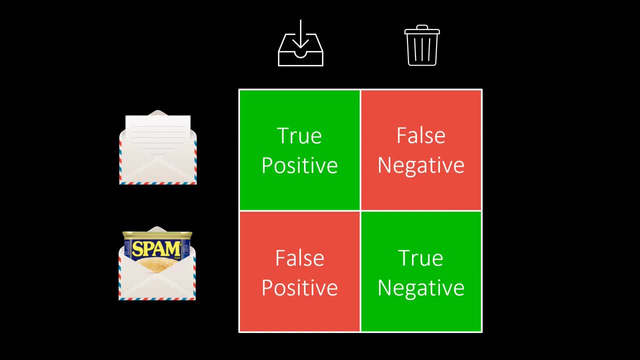 as the prediction of the classifier aligns with the true class of the email. When the email is legit and our classifier correctly classifies it as legit, we have a so-called true positive. When the email is spam and our classifier correctly classifies it as spam, we have a true negative. In contrast, when the email is legitimate, 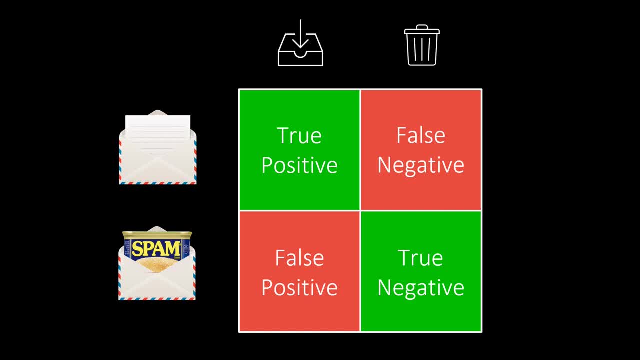 but characterized as spam, we have a false negative. And when the email is spam and our classifier mistakes it for a legitimate email, we have a false positive. This matrix is interesting by itself, and we usually write in each cell how many cases of 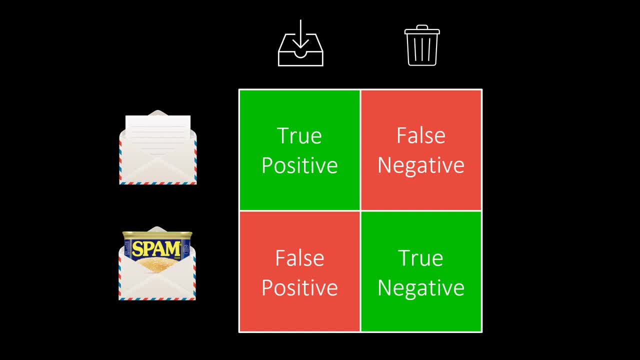 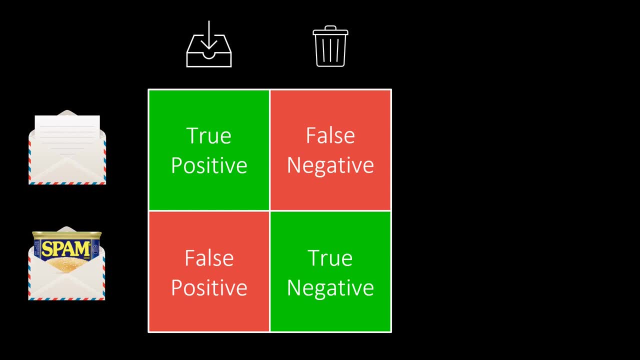 this combination we have seen in our training or evaluation set. We can also define a variety of metrics to characterize how our classifier performs. One such metric is the accuracy, which measures the number of true positives and true negatives as a fraction of the total number of predictions. 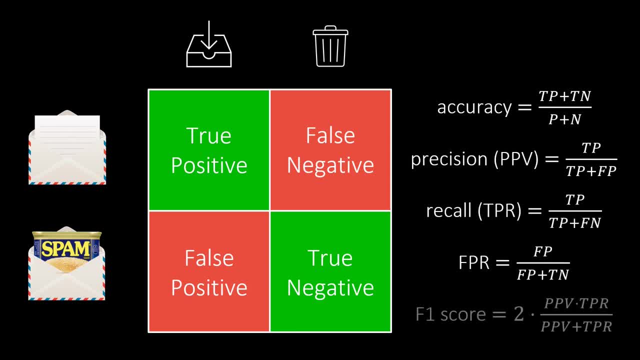 However, we can also define the accuracy of the number of true positives and true negatives as a fraction of the total number of predictions. We can also have other metrics, such as the true positive rate, which measures the number of true positive predictions as a fraction of the true positive. 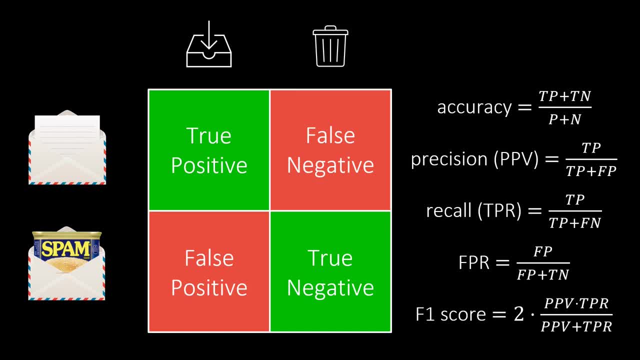 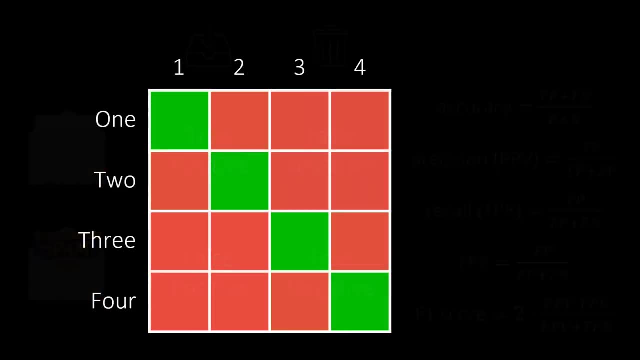 and false negative predictions and the false positive rate, which measures the number of false positives as a fraction of the false positive and true negative predictions. Here are some of the most common ways to express the quality of a classifier with a single value. We can also extend this analysis beyond two classes. 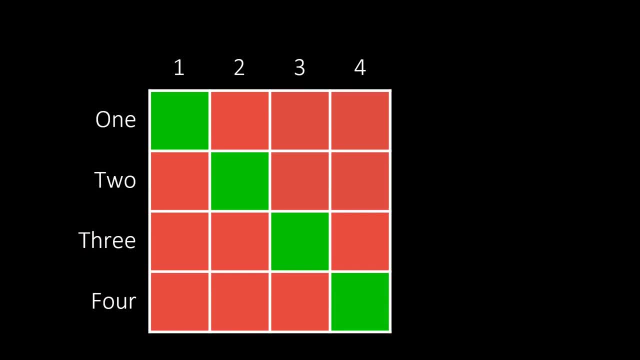 In this example, we want to learn to understand spoken versions of the digits from one to the other. We can also extend this analysis beyond two classes. We can also extend this analysis beyond two classes. We have four classes and four possible predictions, so we get a four-by-four matrix. 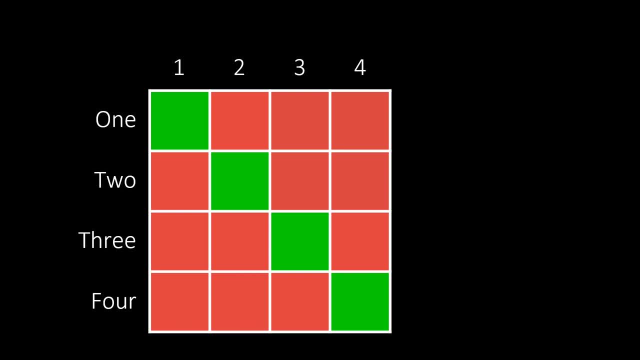 The combinations where real types match. the classifications are in the diagonal. These green cells are all the good combinations where we classify correctly. The red cells are incorrect classifications. Such a matrix is called confusion matrix. Evaluation can also help us to understand the hyperparameters of our classification algorithm. 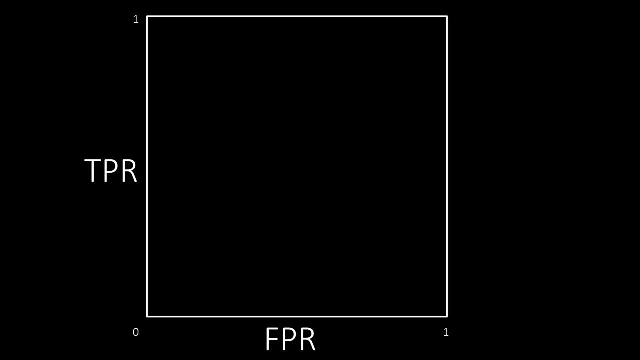 For instance, in the case of a binary classifier like our spam filter, we can decide how aggressively we want to classify an email as spam. If our classifier categorizes all emails as legitimate, our true positive rate becomes 100%, but so does our false positive rate, since we will not have any true negatives or false negatives. 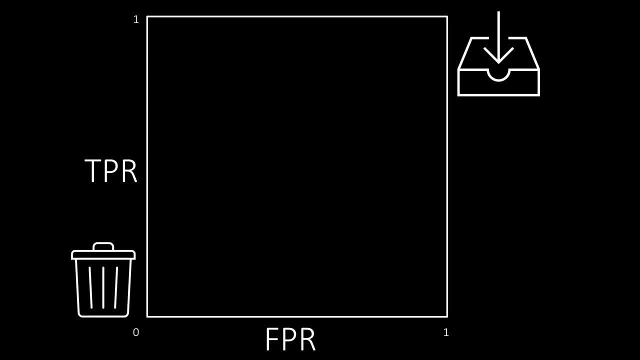 On the other hand, if the spam filter classifies all emails as spam, both our true positive rate and our false positive rate become zero. In between these two extremes, we can achieve different combinations of the true positive rate and the false positive rate. 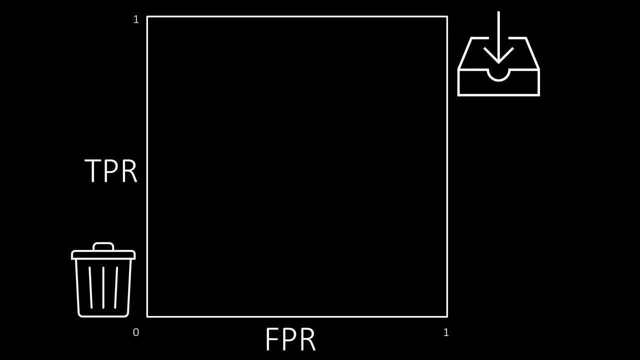 based on how good our classifier is. This is visualized by the so-called receiver operating characteristic curve, or short ROC curve. The ROC curve plots the true positive rate against the false positive rate for different levels of aggressiveness on the x-axis. On the right side, we have the case where the classifier classifies all emails as legitimate. 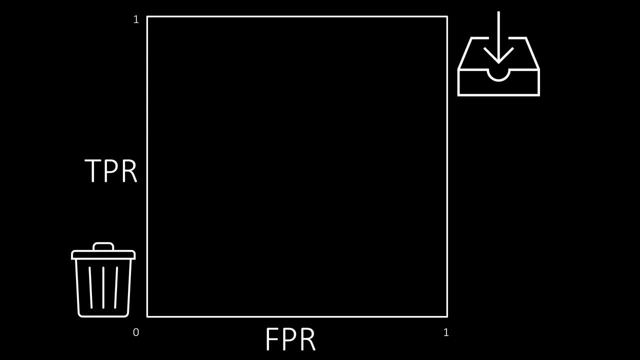 On the left side, we have the case where the classifier classifies all emails as legitimate. On the right side, we have the case where the classifier classifies all emails as legitimate. Can you guess the ROC curve for a completely random classifier? Please pause the video and think about this for a second. 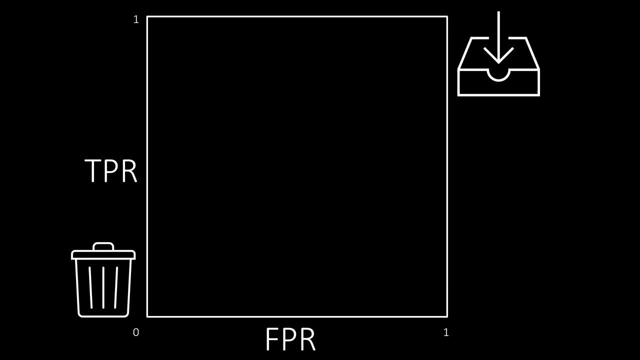 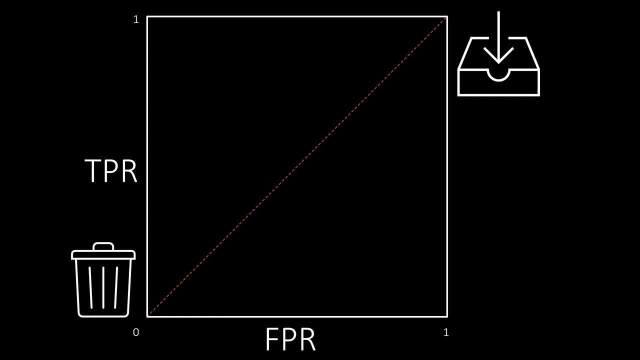 So the curve of a random classifier is just a diagonal line from bottom left to top right. A good classifier will hopefully be above this diagonal. Indeed, the better the classifier, the more it hugs the upper left corner. The upper left corner achieves a 100% true positive rate.